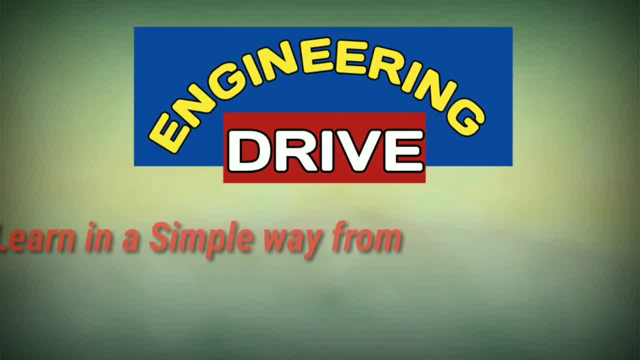 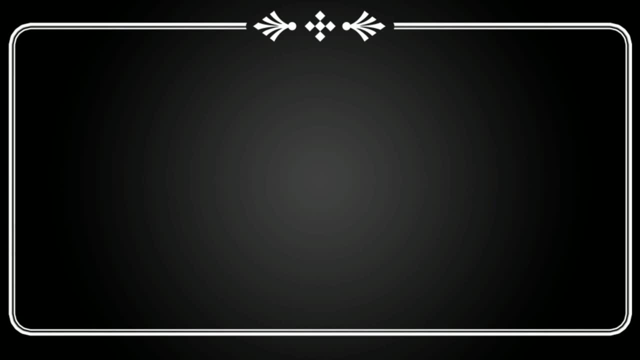 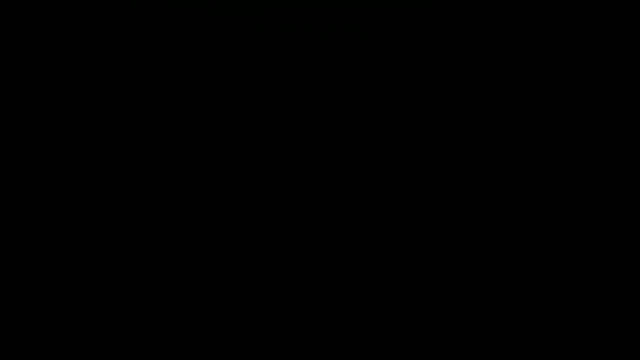 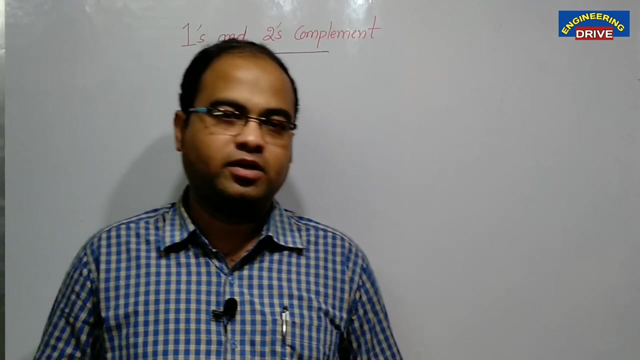 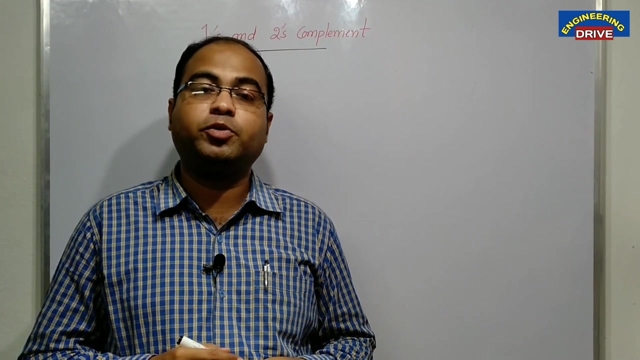 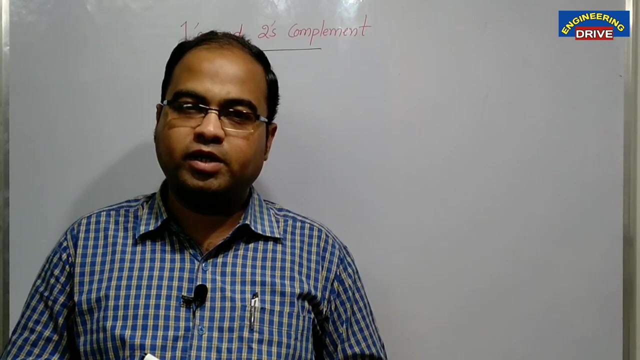 Hi everyone, this is Atik. Welcome to my channel, Engineering Drive. Today I am going to discuss one topic: once and twos complement. Actually, this topic belongs to a series of videos on computer organization subject and why. we will find out. once and twos complement of a number. 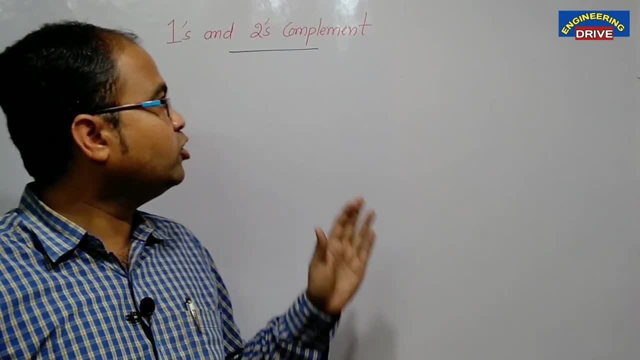 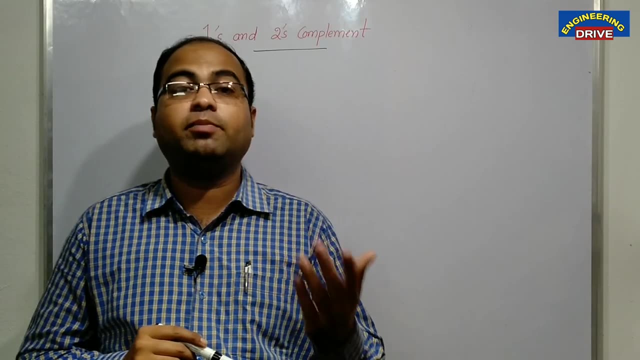 on which number this concept will be useful. If you want to find out once and twos complement, then we need to take a binary number. Once and twos complement can easily be determined on a binary number only If you have not watched how to convert a particular decimal number into binary. 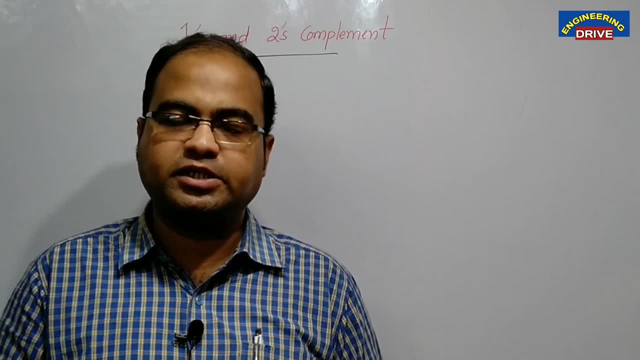 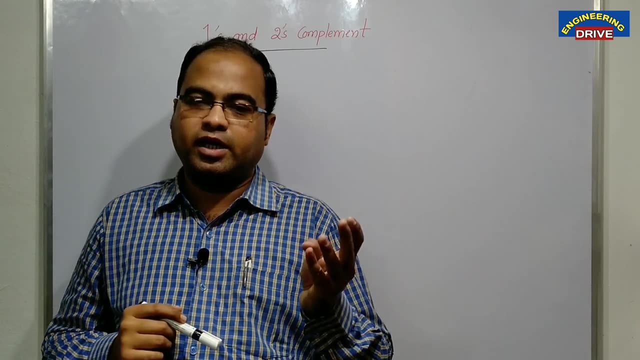 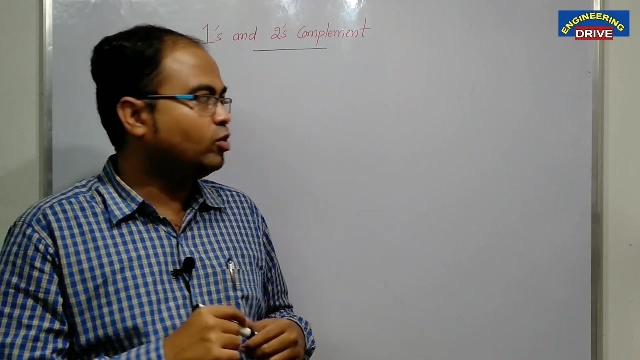 always, you can go ahead to my playlist, computer organization, In that you can find one video titled number systems There. already I have discussed how to convert a binary number to decimal, decimal to binary octal, hexadecimal. everything you can get in detail. Okay, now coming. 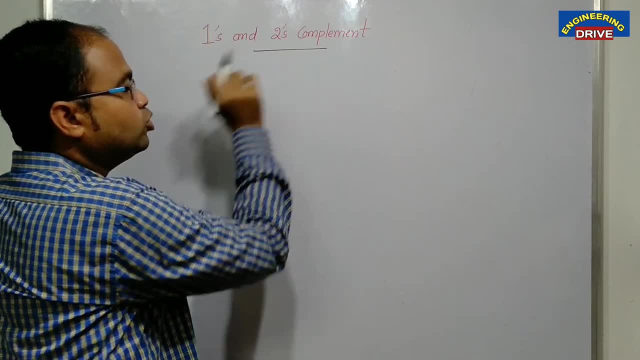 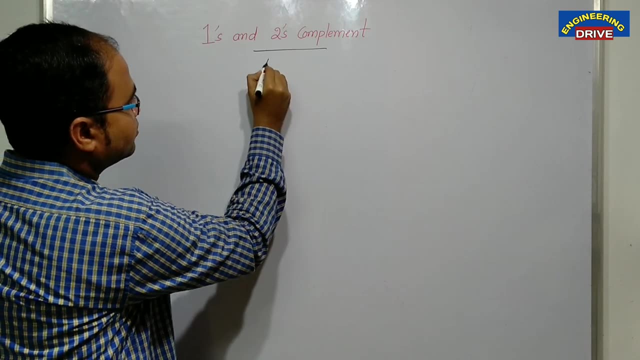 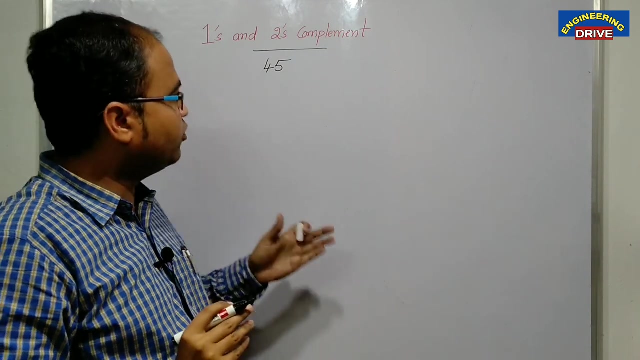 to this today's topic: how to find out once and twos complement and what are the uses of this We will see now. Let us take a decimal number: 45. Okay, I want to find out once and twos complement of this number. So before that, I need to convert this number into binary. So how? 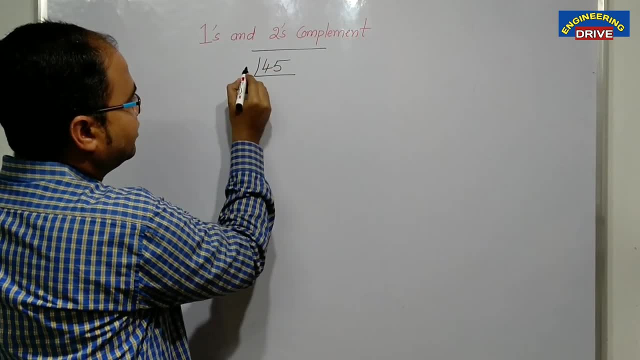 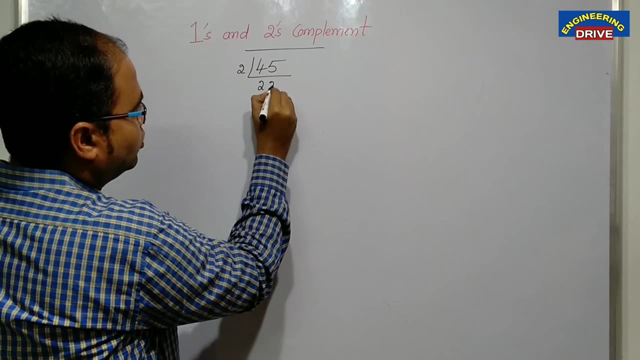 to convert this 45 into binary, Let us divide it with 2, because a binary number have radix 2.. That's why I have taken 2.. 2,, 2,, 22.. How many number will remain? One number, because 45 minus. 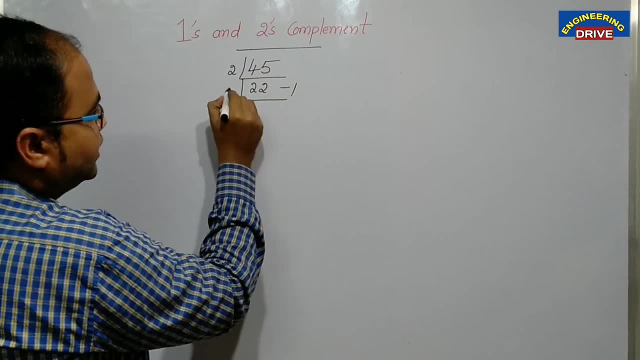 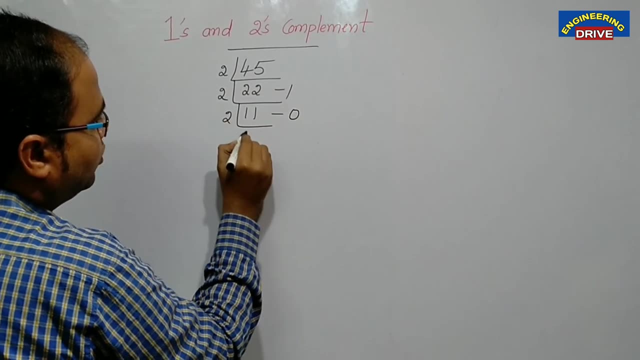 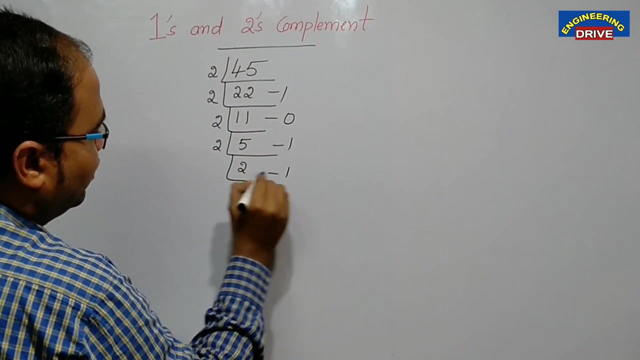 42.. Sorry, 45 minus 44, 1.. Next, 2, 1.. Any number will remain No. Next, 2, 5, 10.. Any number will remain 1.. Next, 2, 2, 4, 1.. 2, 1, 0.. No number will remain. Now, what is the binary form of 45?? 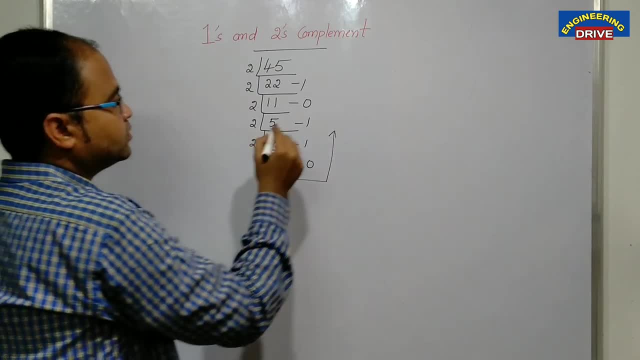 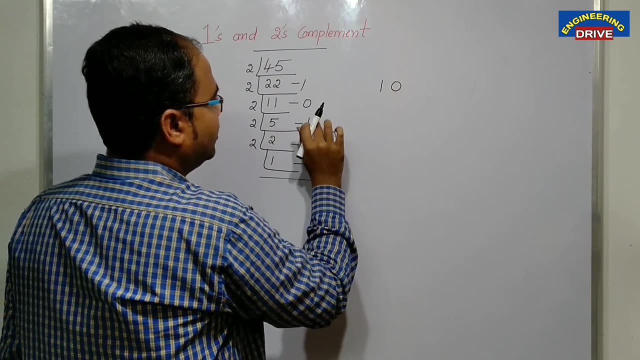 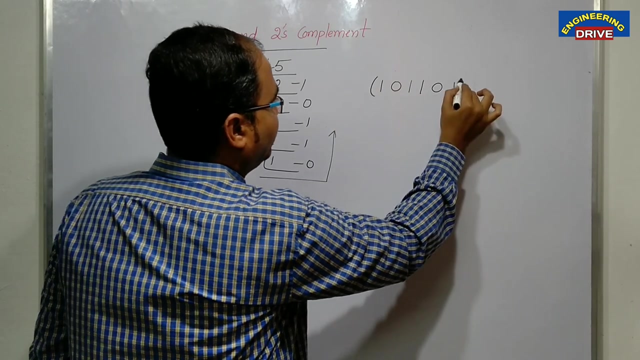 The binary form of 45 is, right down from bottom to top, 1, 0, 1, 0, 1, 1, 0, 1, 1, 0, 1.. So this is the binary form of 45.. Now I want to find out once and twos. 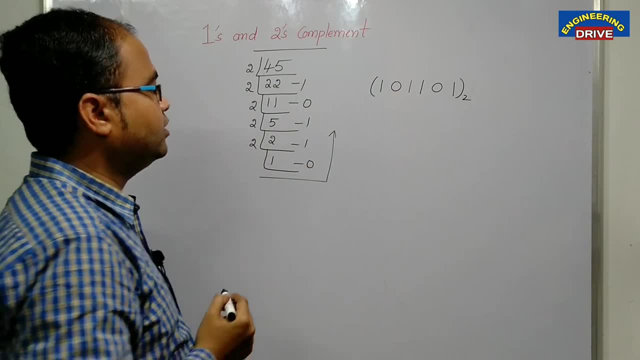 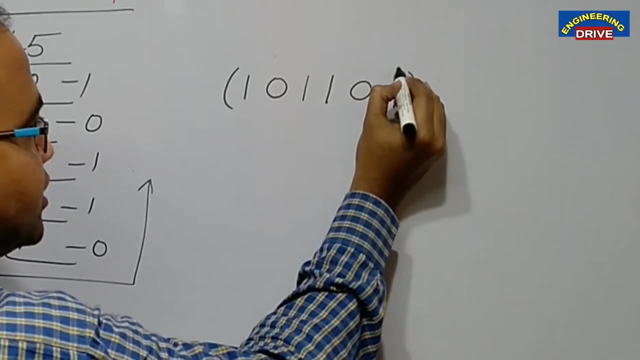 complement of this binary number. How to find out once and twos complement. Before that, let us check whether we got answer correct or not, Whether it is the binary number of 45 itself. How to cross check? Just you keep 1,, 2,, 4,, 8,. 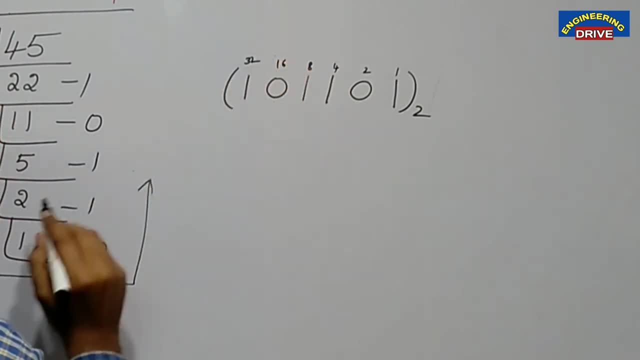 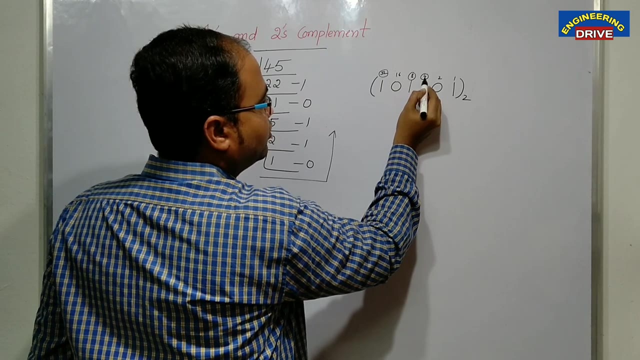 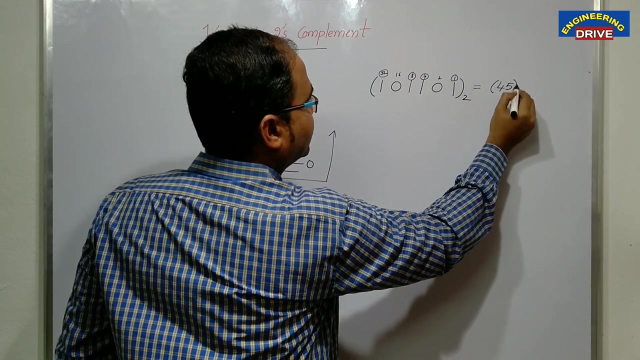 16, 32.. Wherever ones are there, you add: So 32 plus 8 plus 4.. 32 plus 8, 40.. 40 plus 4, 44. Plus 1, 45. So answer is correct. Just cross check method, this one. Now I want to find out once and twos. 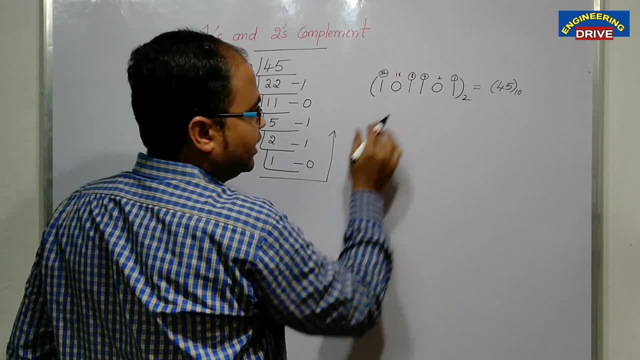 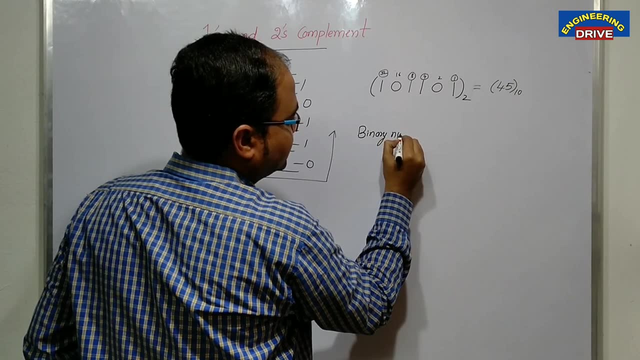 complement. now for this binary number. Let us write down the binary number as it is Now. our binary number is the binary number of 45. is what is a binary number? 1, 0,, 11,, 00,, 1.. 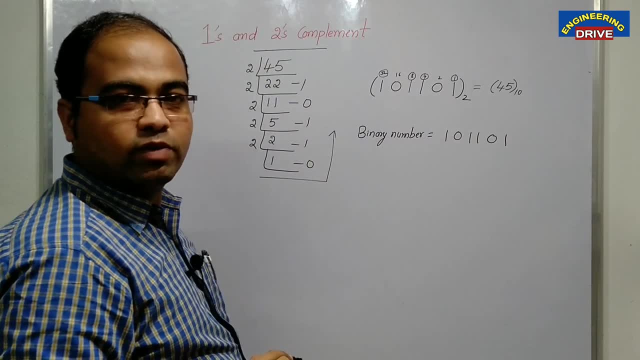 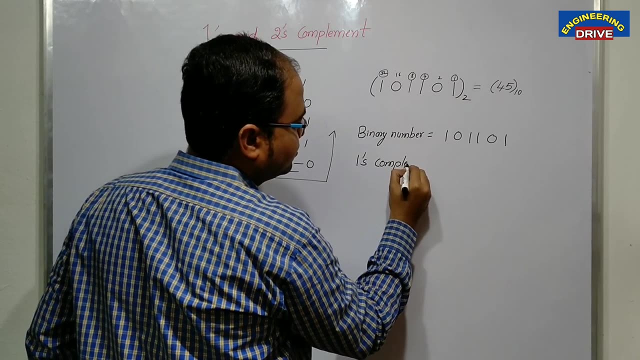 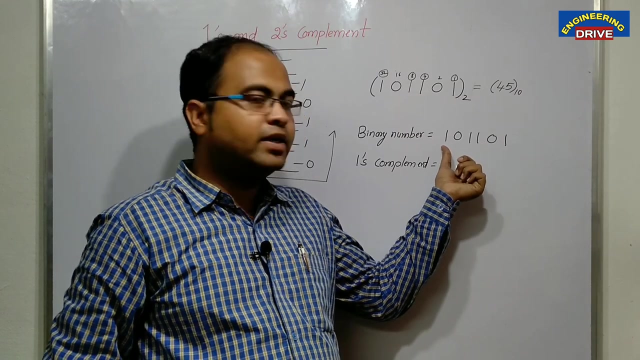 How to find out one's complement. once complement Can be found out very easily by using a simple method. What you need to just reverse the bits Wherever one is there, right zero, wherever x, 0 is there, And then if you turn the earth square then it would have got virtual organisation. 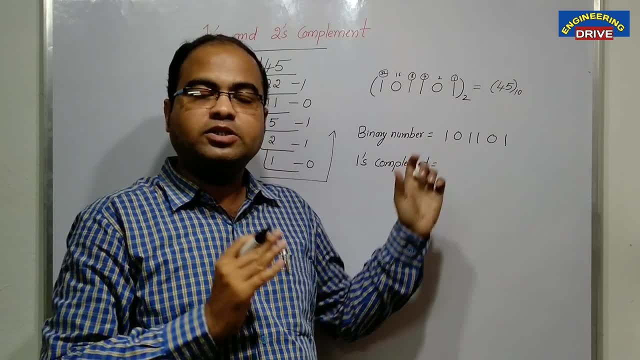 Just to reverse the bits. wherever one is there, right Zero. Whatever one is there, will study it at midnight and willagem the same. So if you want to replace the element and하u willerve and vanñare is there, write 1.. 1's complement of a binary number can be determined by reversing the bits. 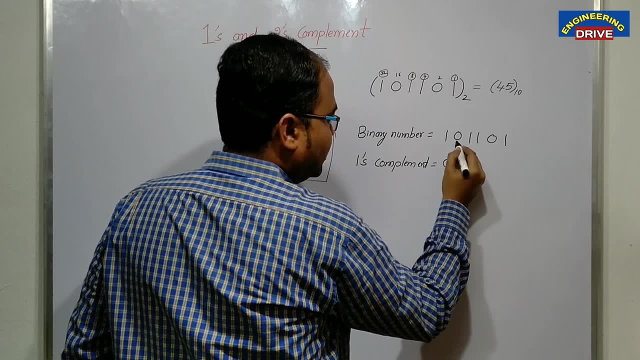 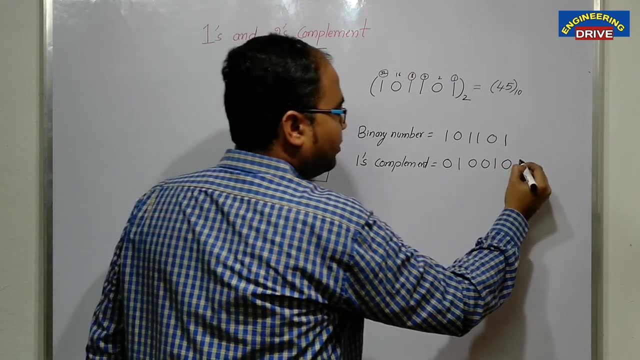 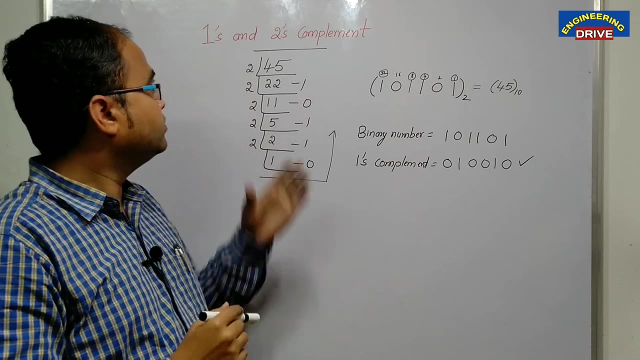 So here 1,, which means you write 0, 0, 1, 0, 0,, 1, 0. So this is the 1's complement of the binary number. So 1's complement is determined by simply reversing the bits. Now 1's complement.